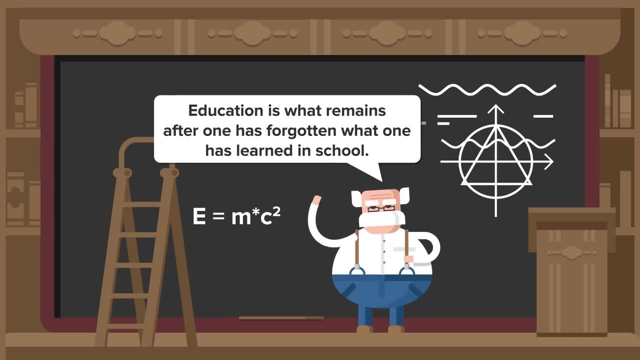 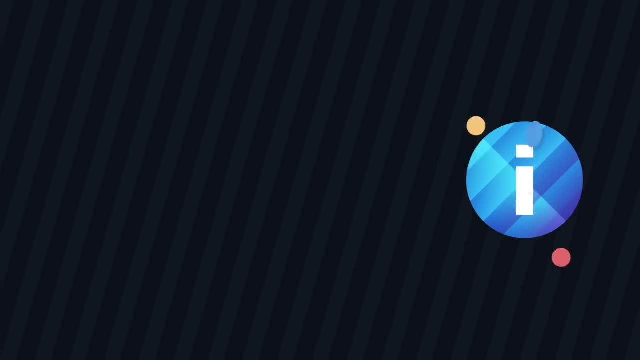 too keen on school. One of those minds was Albert Einstein, who famously said: Education is what remains after one has forgotten what one has learned in school. So does it matter where you go? That's what we'll find out today in this episode of 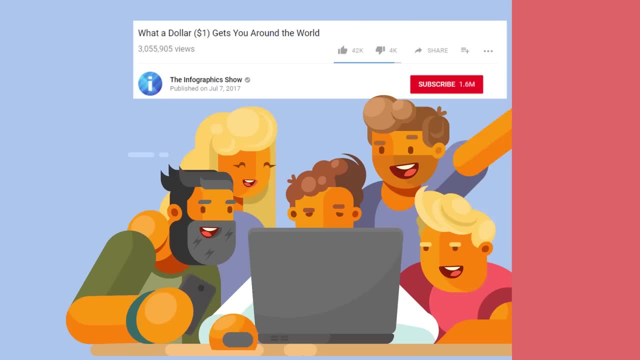 the Infographics Show: Private School vs Public School. Don't forget to subscribe and click the bell button so that you can be part of our notification squad. First of all, we should say that by public school, we mean schools that are run by the 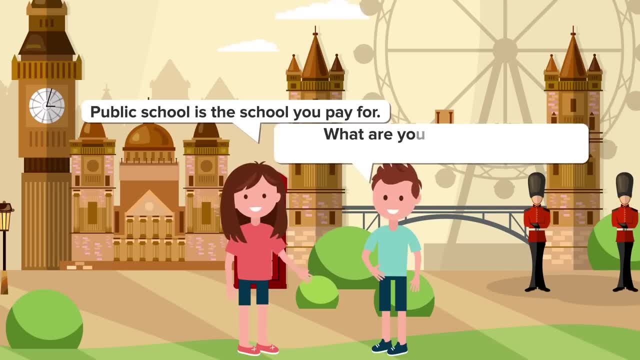 government. This could be confusing for Brits, as when they say public school, they are not thinking of schools run by the public sector, but selective institutions that demand private payment. Basically, private school. as Americans know, it is public school. Public school in the UK. It's another case of tomato-tomato. We'll base this show on 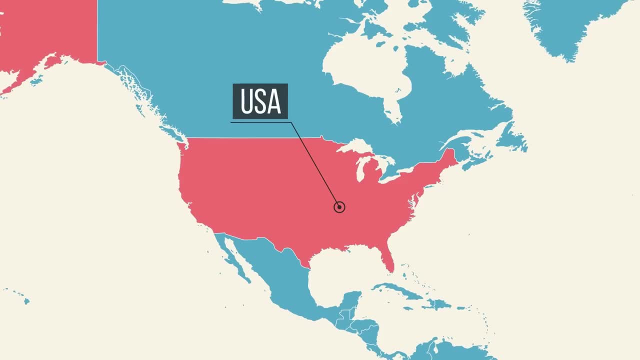 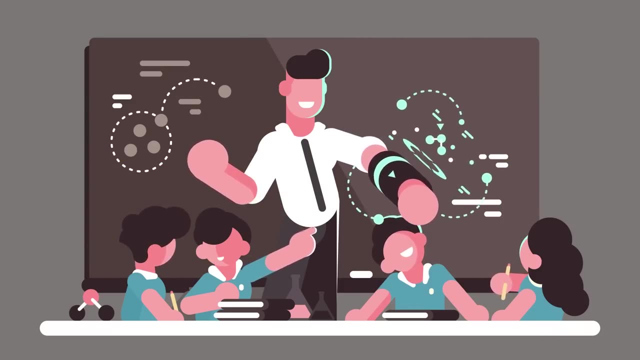 the US today, as covering the globe's schools would be impossible, and some of the things we will discuss are relevant globally. You might be surprised to know that in the USA, according to the Council for American Private Education, there are 33,619 private schools. in the United States, There are around 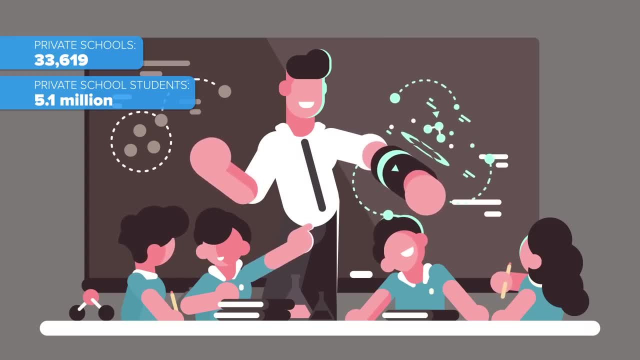 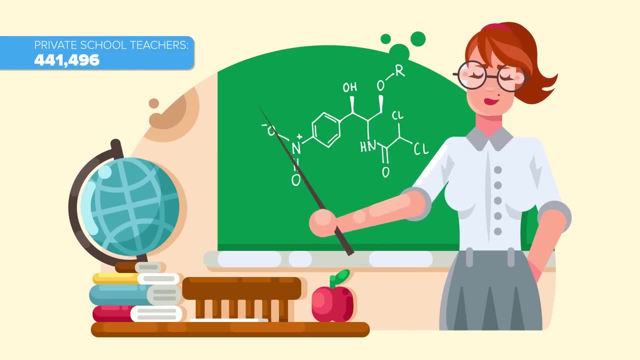 5.1 million students enrolled in these schools. It's said that private schools are home to almost 10% of all school students in the US. The same sources state that there are 441,000 private schools in the United States. There are 496 teachers working full-time in private schools- As much as 79% of these schools. 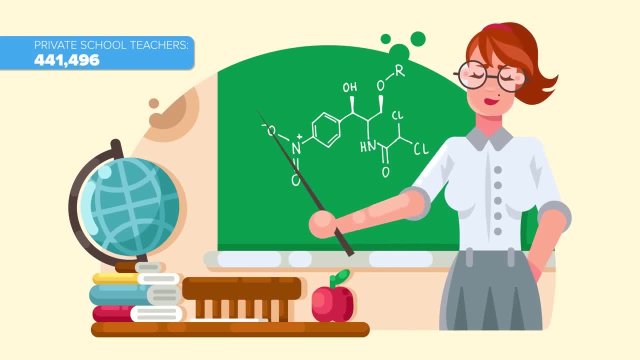 have a religious affiliation. the Washington Post reported in 2016 that these schools are virtually all white, with non-white students only making up around 10% of students across the country. As for public schools, according to the National Center for Educational Statistics, 50.7 million. 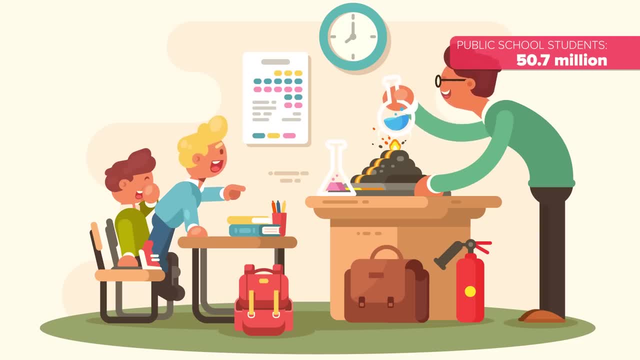 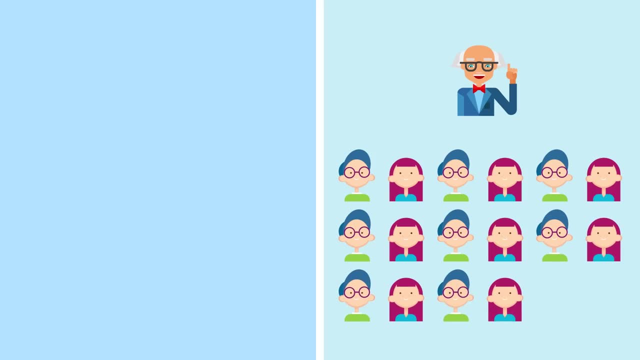 public school. students will be studying in one of them from pre-kindergarten to grade 12 in fall 2017.. Teaching all those kids will be 3.2 million full-time teachers, which is a ratio of 16 students for every teacher. The ratio in private school is 12 students. 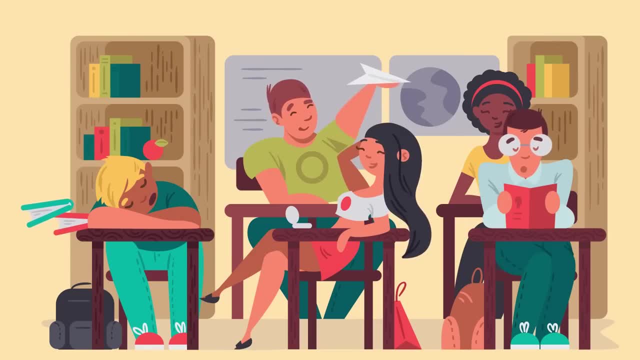 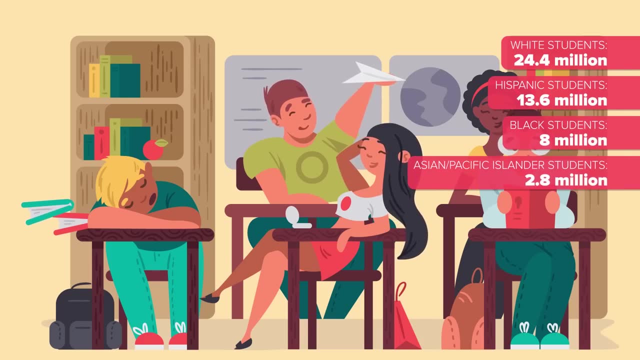 for one teacher. One of the main differences of public school is the mixed ethnicity of students. Public schools in America are made up of 24.4 million white kids, 13.6 million Hispanic students, 8 million black students, 2.8 million Asian Pacific Islander students, 0.5 million American. 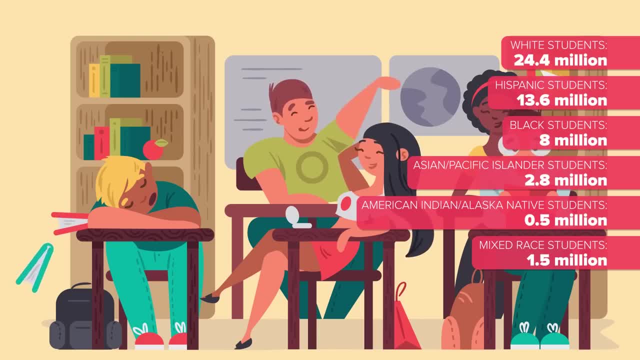 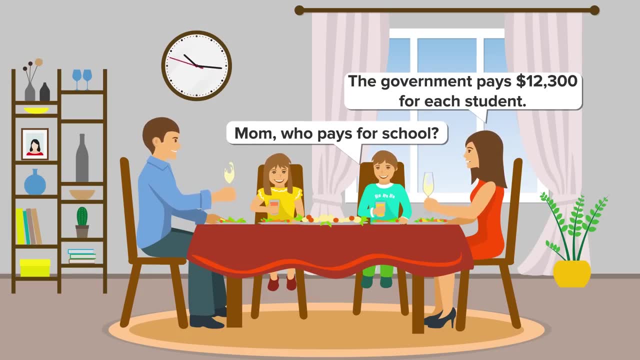 Indian, Alaska Native students and 1.5 million mixed-race students. What about costs? Well, the government pays for public schools In 2020, the government pays for private schools In 2017-2018,. it's projected that the budget for public schools 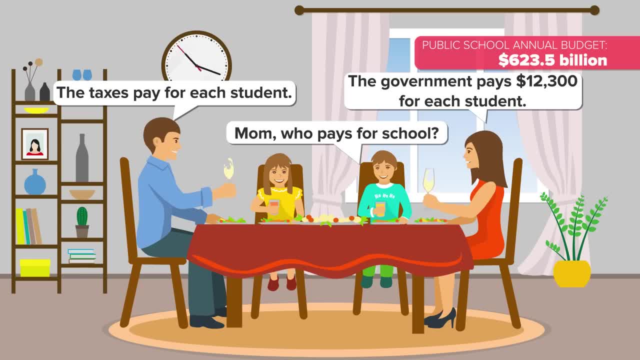 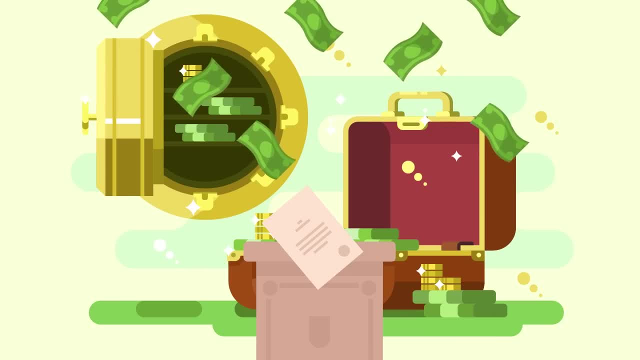 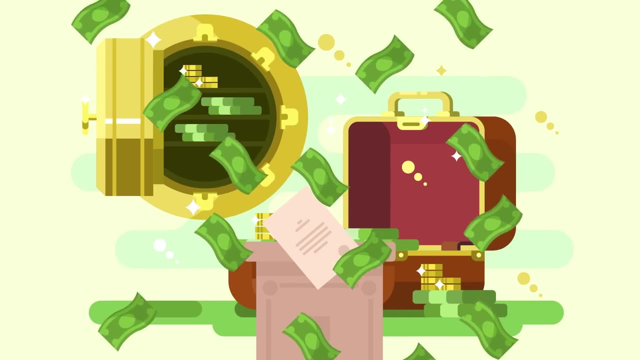 will be $623.5 billion. This means that each student will cost an average of $12,300.. Taxes will pay for this. Private schools are a different matter and they are funded by tuition fees. Tuition costs will change depending on the school. For the year 2017-2018, the national average for private 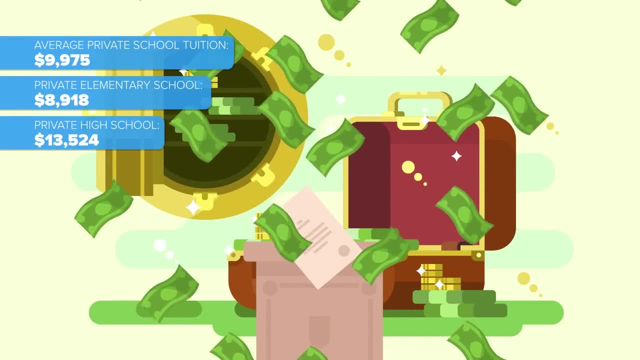 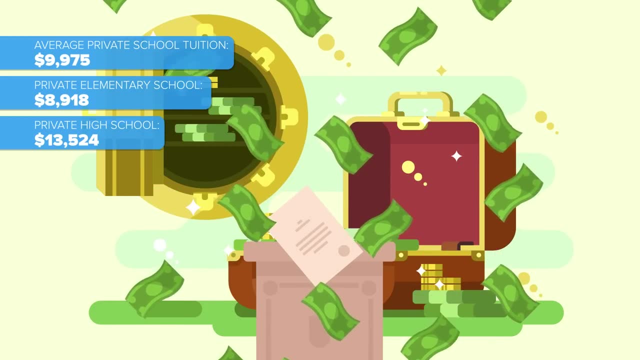 school tuition is $9,975 per year, which is $8,918 per year for elementary schools. For the year 2017-2018, the national average for private schools is $13,524 per year. for high school, The state of Vermont had the highest average, with high school being $31,543. 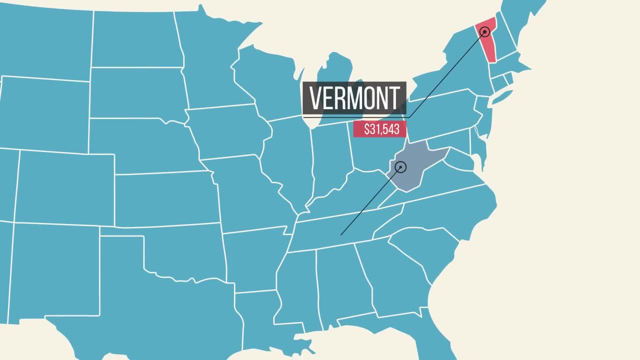 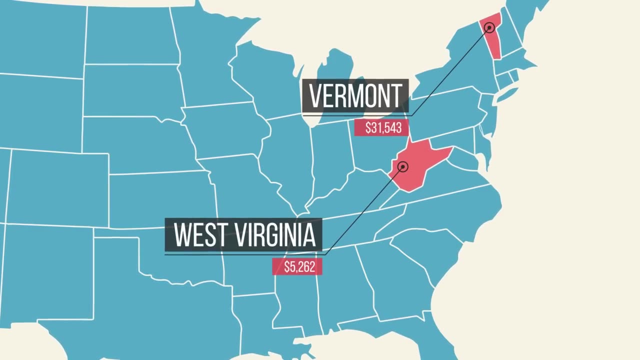 per year on average. If you are looking for cheap private schooling, head to West Virginia, where the average cost for high school is currently $5,262.. We should add that a handful of private schools cost around the $50,000 a year mark. 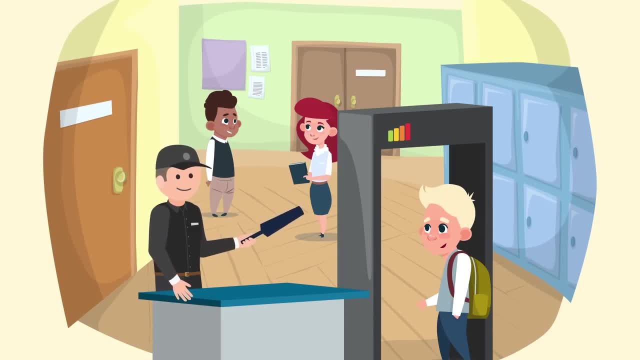 So what do you get for your money besides pretty gardens and, obviously, top-notch facilities at a private school and perhaps metal detectors and patrolling policemen? Well, you can get a $5,000 private school fee, which is about $50,000 a year. 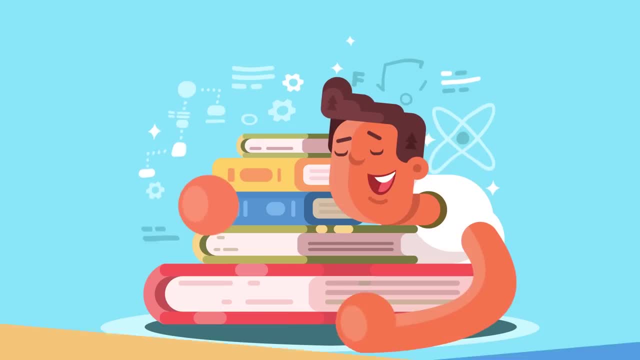 So what do you get for your money besides pretty gardens and, obviously, top-notch facilities at a private school and perhaps metal detectors and patrolling policemen in some wayward public schools? Well, when it comes to the syllabi, public schools have to adhere to state standards. 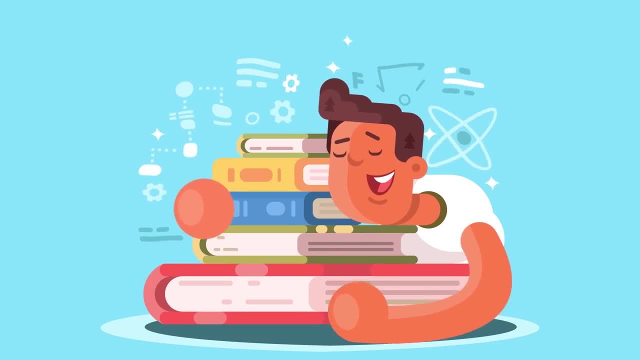 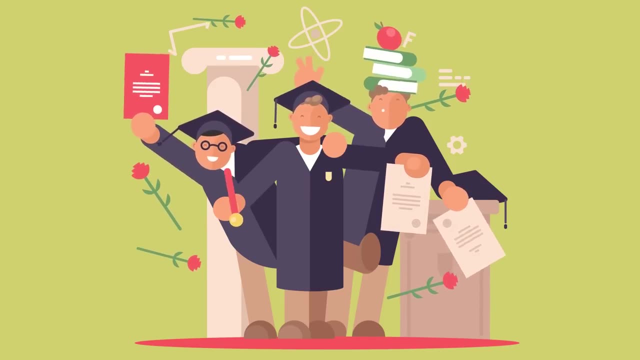 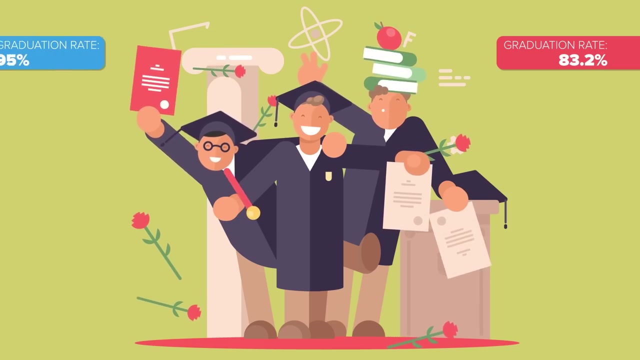 while private schools have much more flexibility. This is seen as getting a better and more diverse education. The good news for not so wealthy people is that high school graduation rates in public schools has gone up recently. It reached its highest during the Obama Administration in 2015, at 83.2 percent of students graduating. At the same time 95 percent of private school. 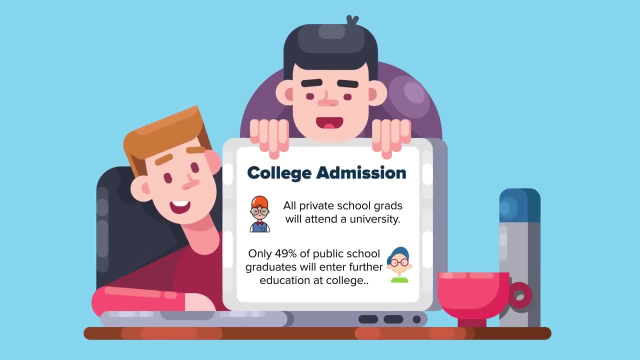 students graduate. According to the website College Admission, just about all of those private school grads will attend public schools, attend a university, whereas only 49% of public school graduates will enter further education at college. If you want to get into an Ivy League university, there's no reason why you can't get in. 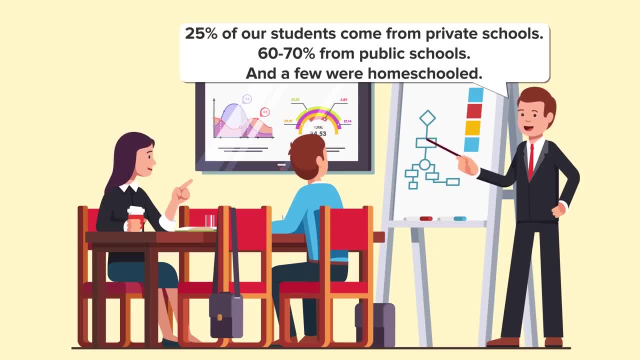 after attending public school. Top-tier admissions tells us that roughly 25% of successful applicants to those top universities came from private schools and 60-70% from public schools. The rest were homeschooled. Private school does work for a lot of people. 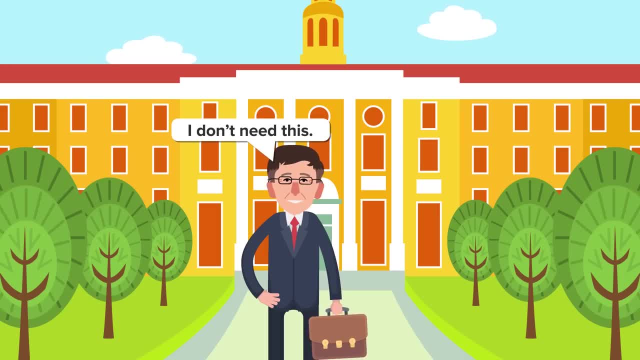 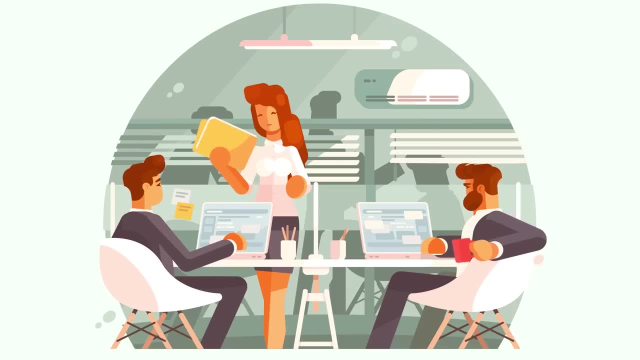 The richest man in the world, Bill Gates, went to a private prep school, but then he later dropped out of Harvard. On the other hand, Facebook founder Mark Zuckerberg went to a public school. When researching for how private school graduates out-earn other kids in the future, most of 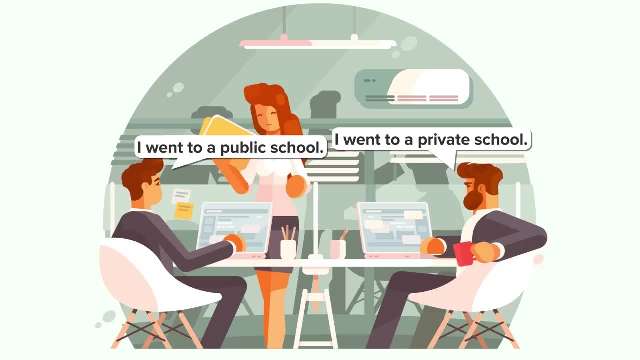 the stories are about the UK and how private school there seems to create most of the UK's millionaires. The US playing field might be a bit more level. after all, Dr Dre didn't go to private school. It seems in the US, if you actually get to university, it might not matter where you. 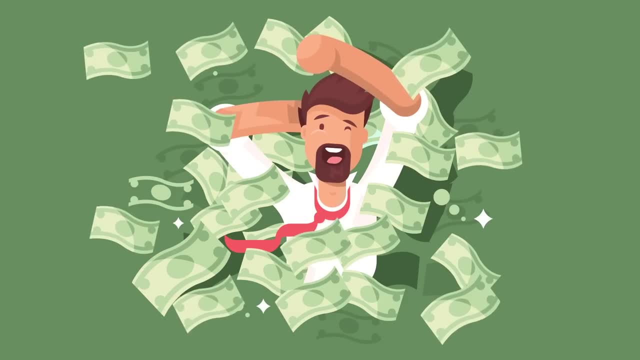 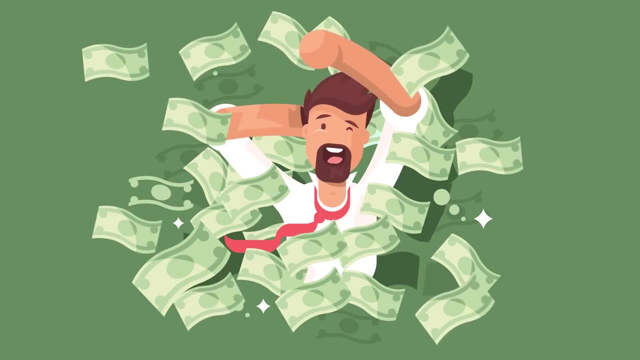 studied in high school in terms of making it. At the same time, studies have found that being born with a silver spoon usually means you'll be passing that spoon on. Even poorer folks with degrees don't usually jump up a class. Your background makes all the difference. 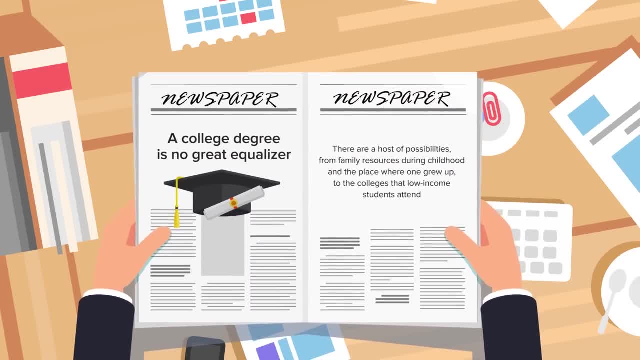 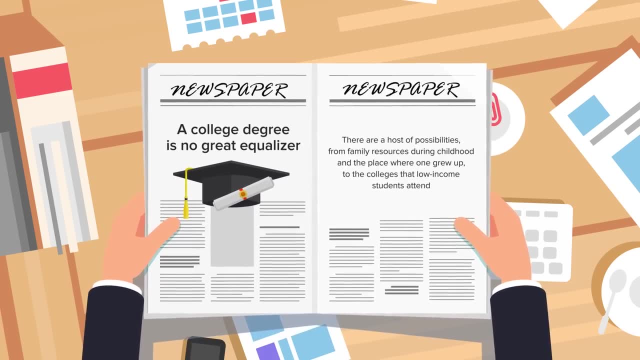 A college degree, says one report, is no great equalizer. Why is this? There are a host of possibilities, from family resources during childhood and the place where one grew up to the colleges that low-income students attend, said their report. 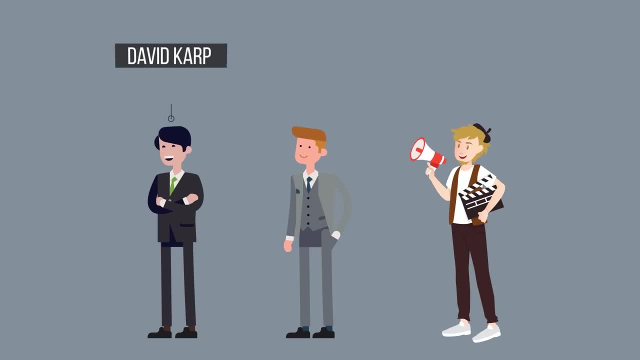 Then you have rich folks that dropped out of high school, such as the billionaire Tumblr founder, David Karp, who dropped out of high school at 15 years old. Joining him as a high school dropout is Facebook's former product manager, Mike Hudak, and filmmaker. 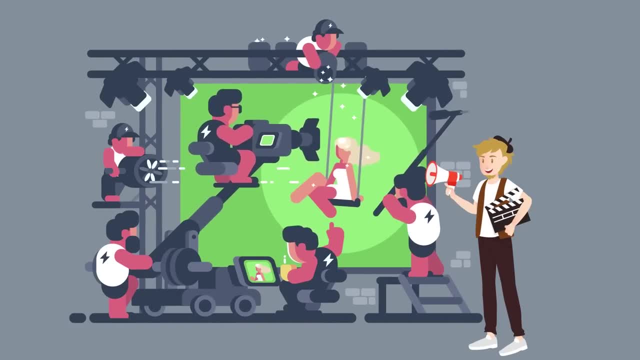 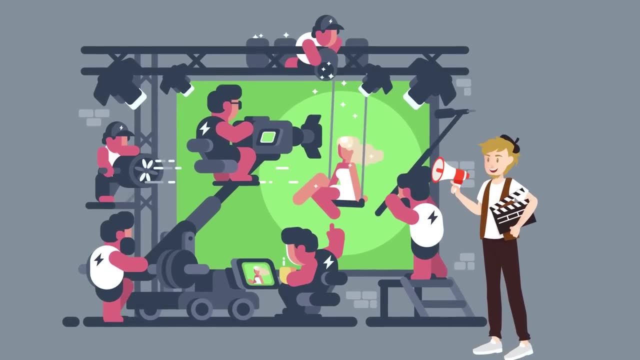 Quentin Tarantino. In light of the last person, success in the arts or sport probably is not related to if you went to public or private school, but if you want social mobility then it's probably better. your parents paid the cash for your education. 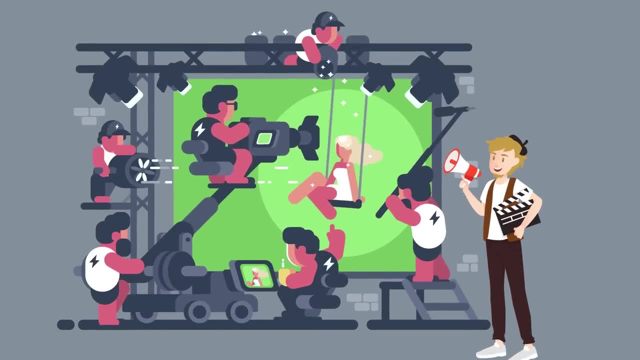 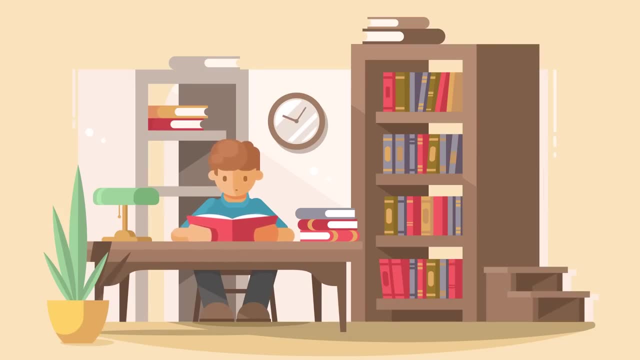 It also seems that the filmmaker is the only one of the three to have come from a humble background. You may have some unique skills or be a natural autodidact, and so school doesn't matter much, even if you are poor. Nonetheless, we can't ignore some statistics. 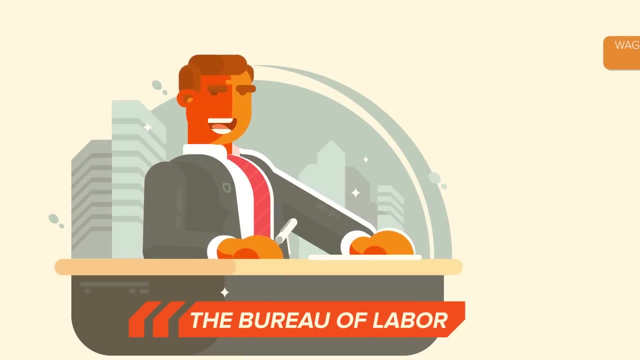 The Bureau of Labor Statistics states that people without a high school diploma will earn, on average, $10,000.. The average is $25,636 per year if in full-time employment. 8% of high school dropouts are currently unemployed. 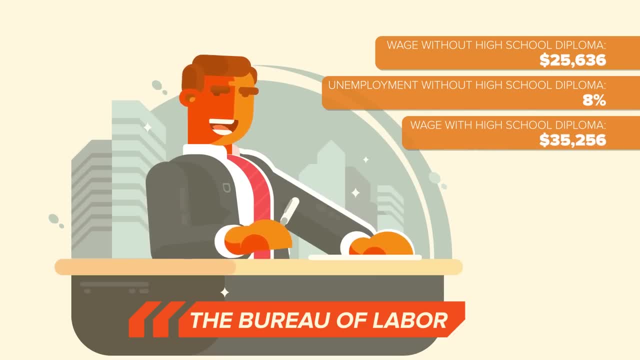 If you have a high school diploma and nothing else, the average wage is $35,256 per year, with 5.4% of those people currently unemployed. If you have a bachelor's degree, you might earn an average of $59,124 per year. 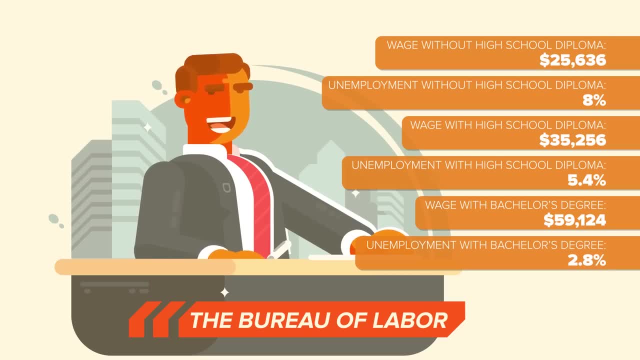 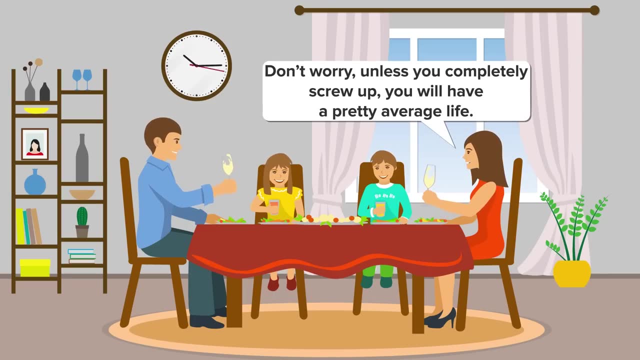 Only 2.8% of Americans with a bachelor's degree are unemployed, much less than the 4.4% of Americans currently out of a job. In conclusion, it's odds on that if you went to private school, then you most certainly. 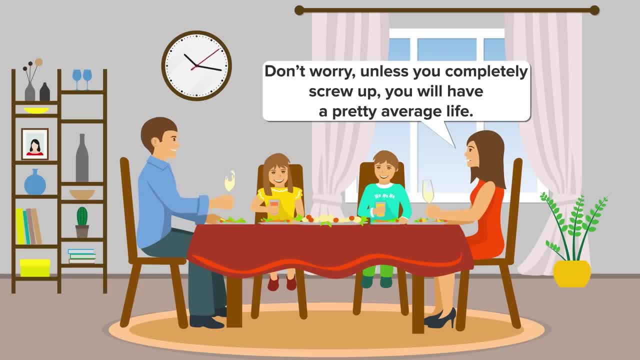 went to university and with some family wealth behind you, it's also pretty much a certainty- you fell into one of those higher wage brackets. Then again, if you are brilliant or spend more time reading than scrolling, then it is likely nothing will hold you back.